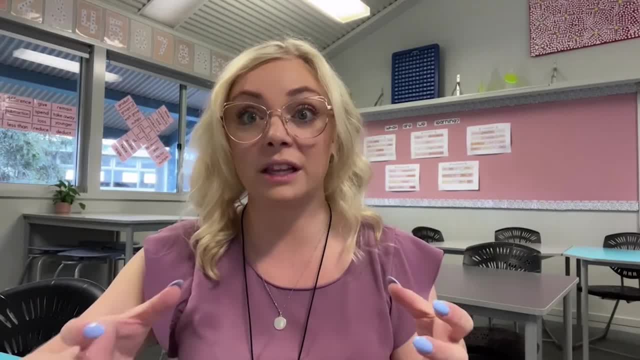 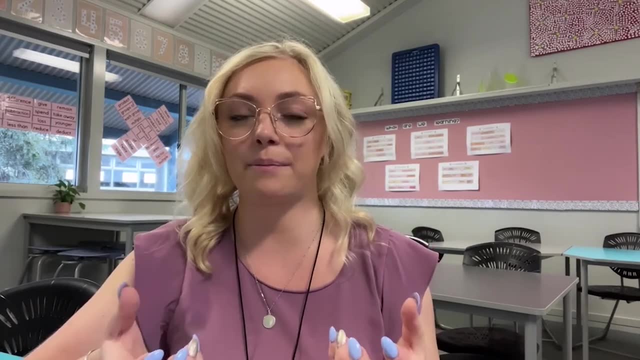 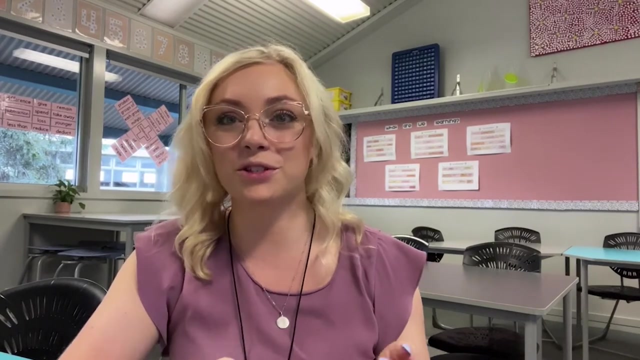 This activity is really great for having students really visualize those unseen parts of their 3D shapes and really get that conceptual understanding happening of moving from that 2D to that 3D shape. This activity, especially when used with students in groups, is really great at promoting. 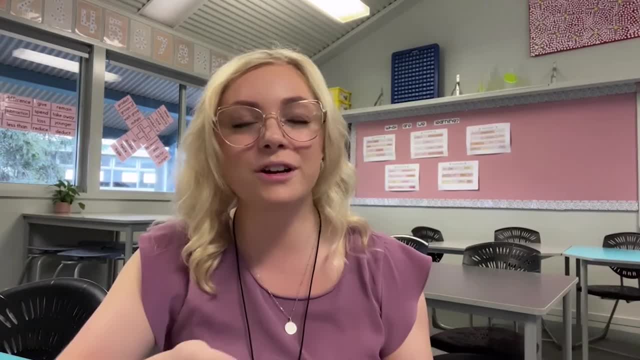 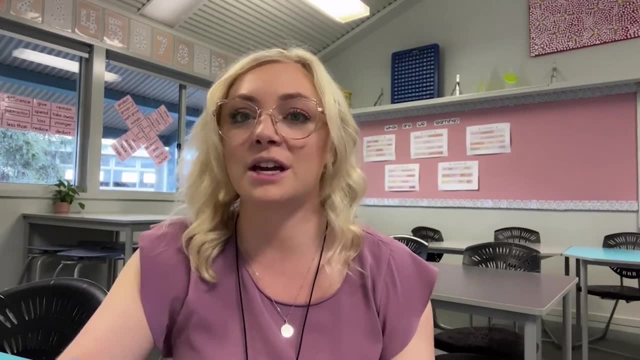 those sort of deep conversations between students and really help them understand the movement from a 2D shape to a 3D shape and how the area and surface area can be used to build that 3D shape. The area of a 2D shape can be the same as the surface area of a 3D shape, and just that movement. 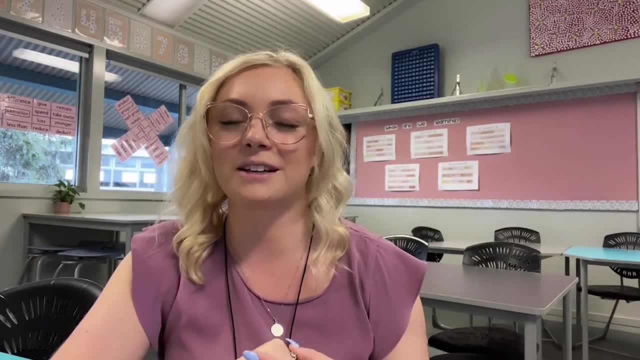 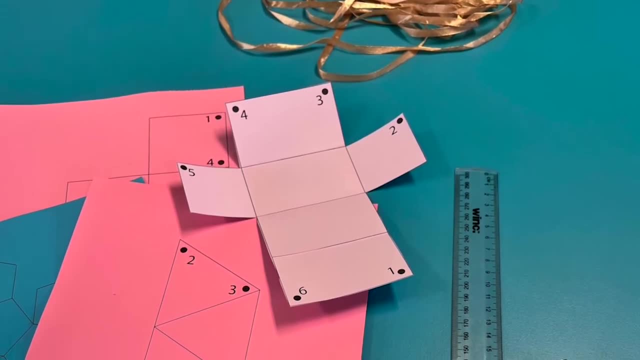 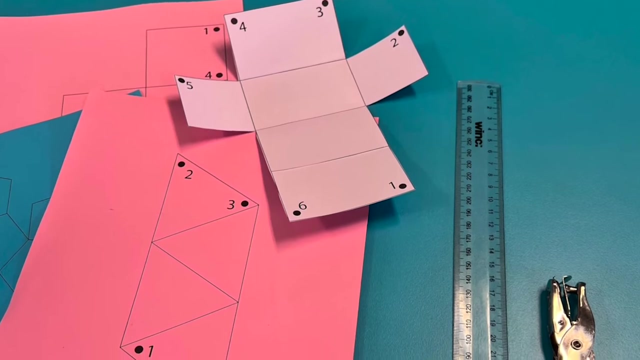 of the of the paper shapes really helps students kind of visualize that To begin this activity with students you do need a few different pieces of material. You of course need the templates which will be linked to this video, a ruler for measuring the size of each of the shapes, a hole punch and 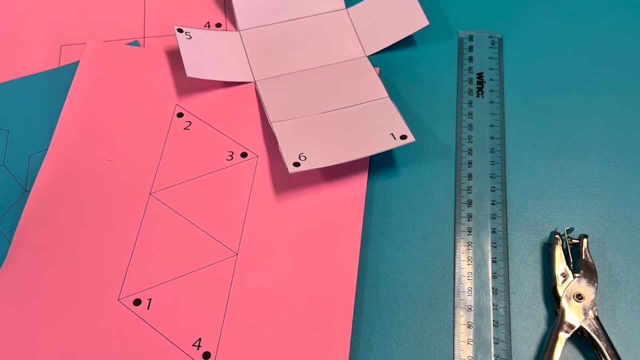 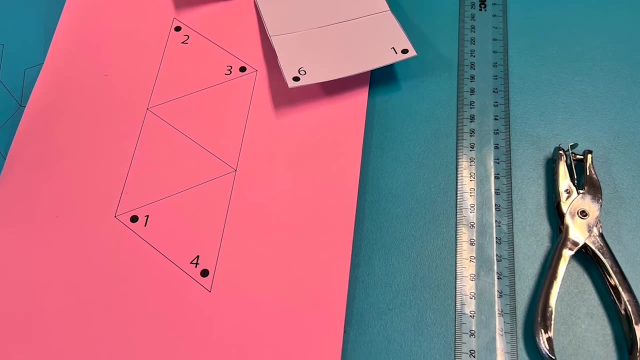 some string. I tend to also grab a glue stick for each of the students so they can glue the base of their shape down onto either a bit of cardboard or into their books, just to make it easier when they are pulling those pieces of string. It makes it so the whole shape doesn't fold in on itself. 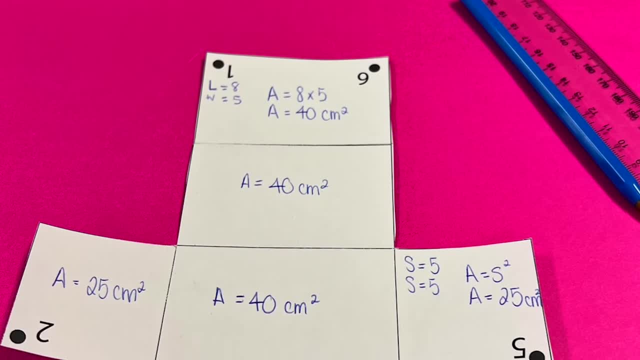 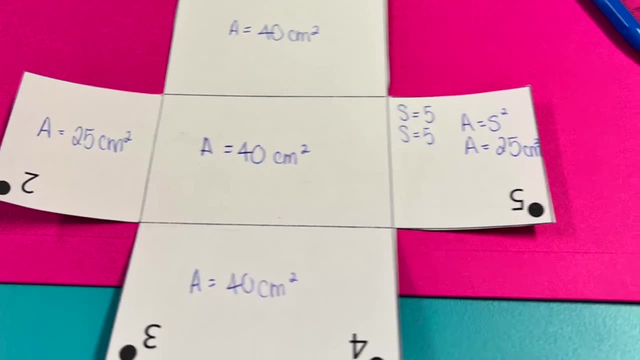 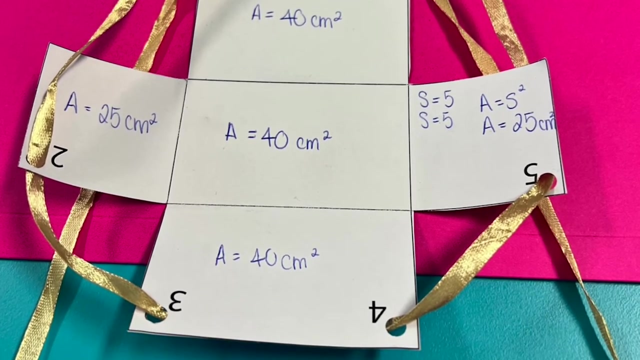 Now, the first step here is to have students measure each of the areas of the shapes and write that total in that box. Now, as you can see here, I am now pulling the bits of string which have been threaded through each of those holes made by the hole punch to make our two. 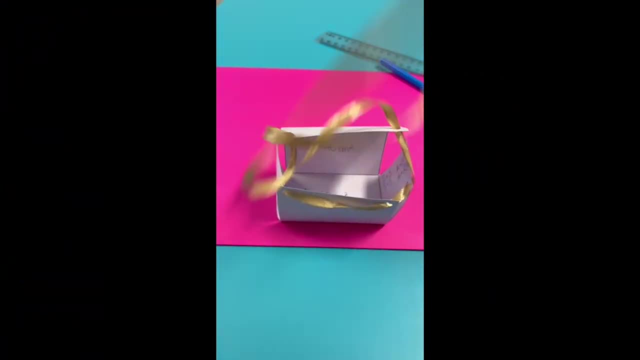 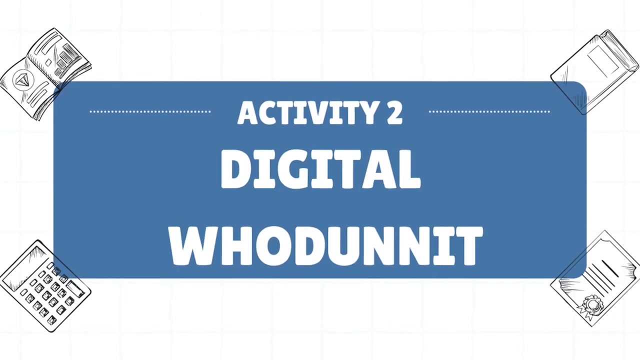 D shape turn into a 3D rectangular prism. Now this is a really nice activity because it's super easy to unfold this one back out to have another look at what the measurements are, or even put the measurements on the outside of the box. This second activity is a digital whodunit, So it's 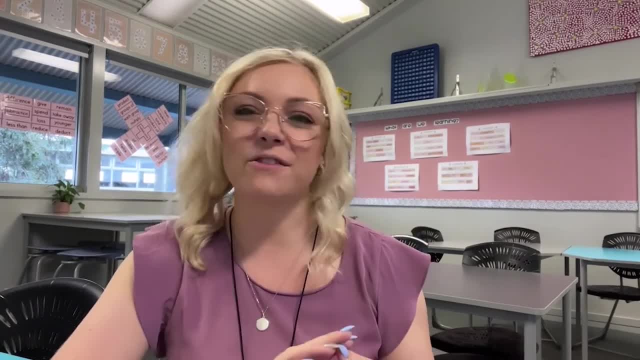 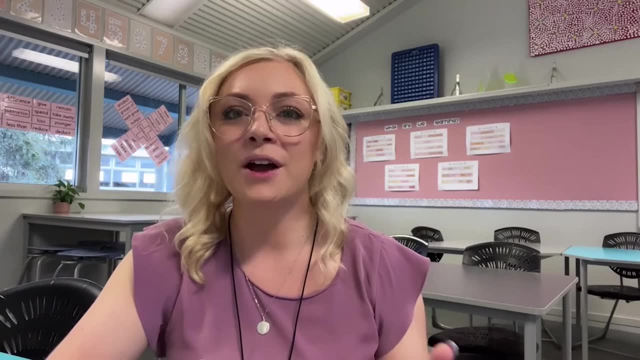 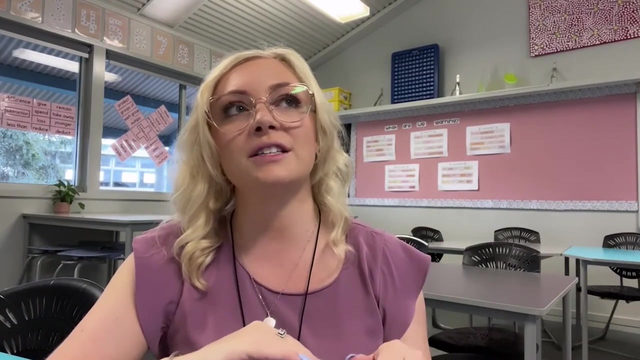 an awesome activity to assign students for homework, if you've got any students working from home or if you wanted to do it in class. it works really well in class as well. So this is a bit of a play on the old Cluedo, so a murder mystery per se, where students have to answer mathematical. 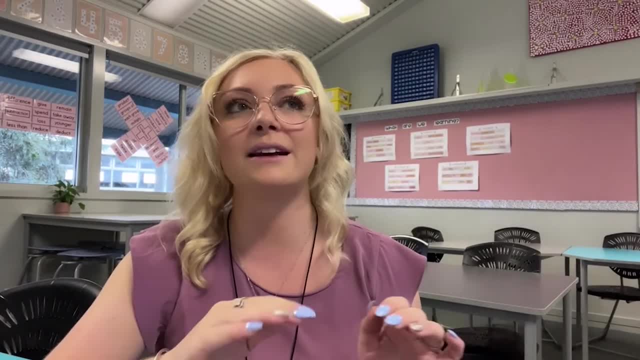 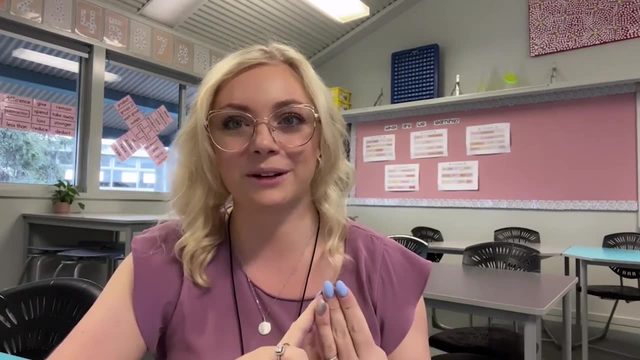 questions to cross off clues and narrow down the person who committed the crime, where they committed the crime and the weapon that it was committed with. This is a Clark creative resource and can be found on their website. They do also have a website where you can find all of the 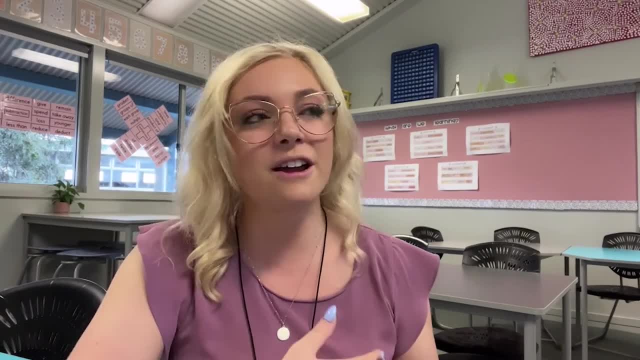 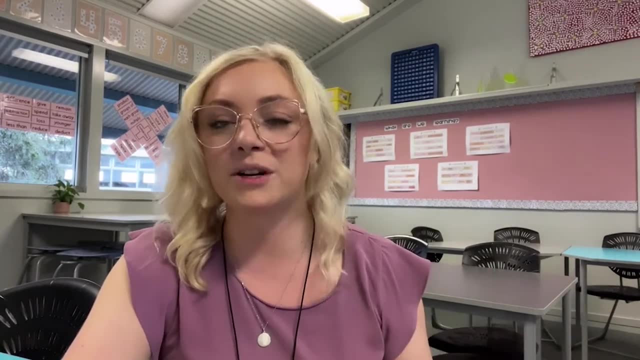 information you need to know about this activity. You can also have printable versions of the same activity as well, So if your students were liked more tactile activities, the exact same activity can be downloaded, printed and set up as a classroom activity as well. I have found that 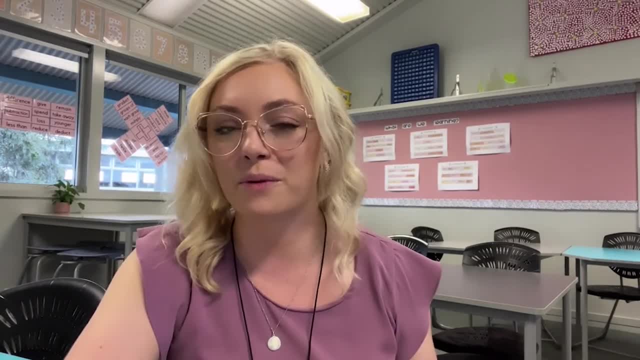 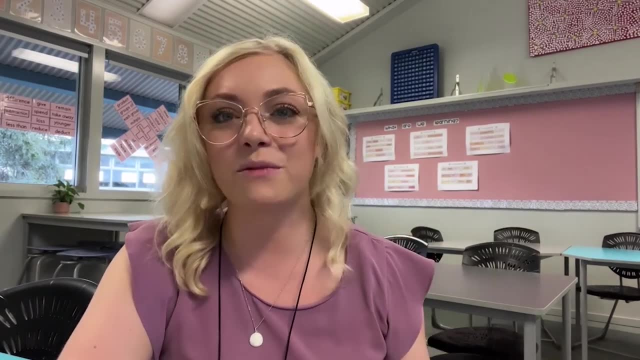 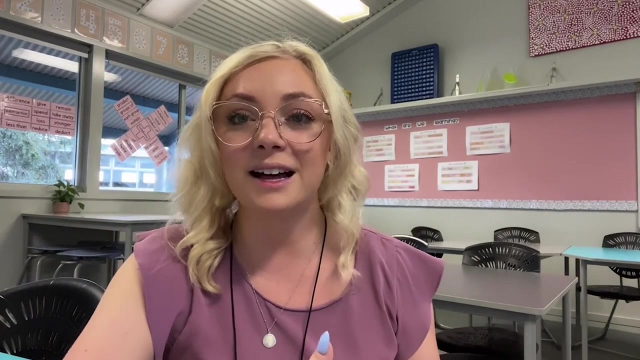 the digital ones are really good for those quick, no prep lessons which really engage the students as well. Usually, what I like to do is assign them through the Google Classroom, creating one copy of the lesson in class, and if, on the off chance, they don't finish it, it's very easy then to move. 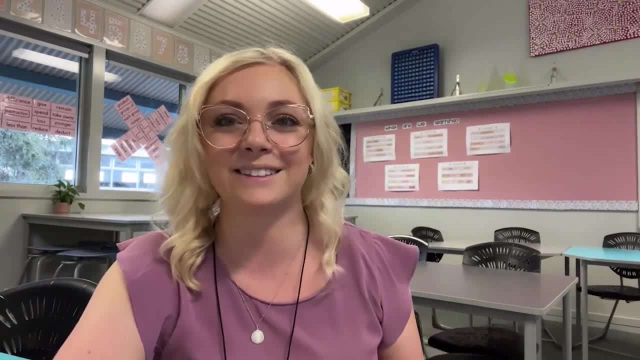 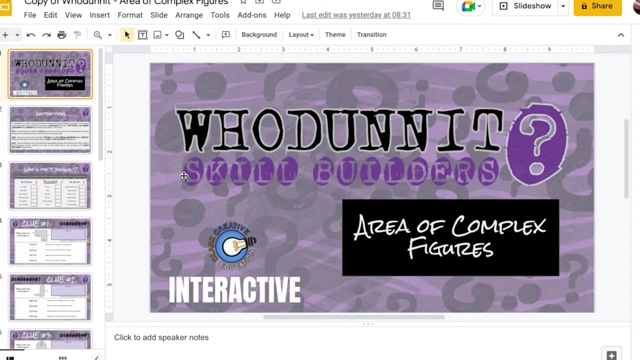 and say, okay, finish this one for homework, because you can access it at home as well. So when students access their copy of the Google Slides, they are initially presented with this whodunit homepage here. This specific one is the area of complex figures, but there are a whole. 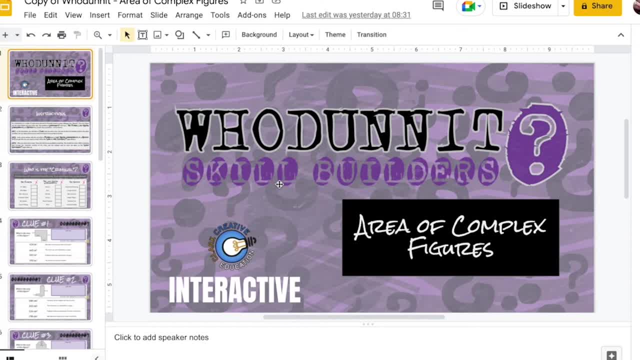 range of them on the Clark creative website, which cover all of the different aspects of the area, surface area, volume and so on, as well as a whole range of other topics as well. So students can then click through the slides on the left-hand side here reading the instructions. 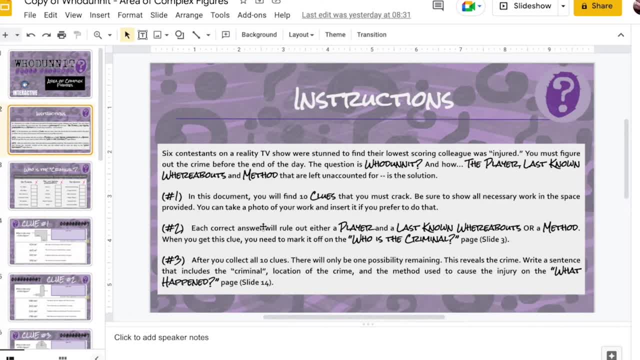 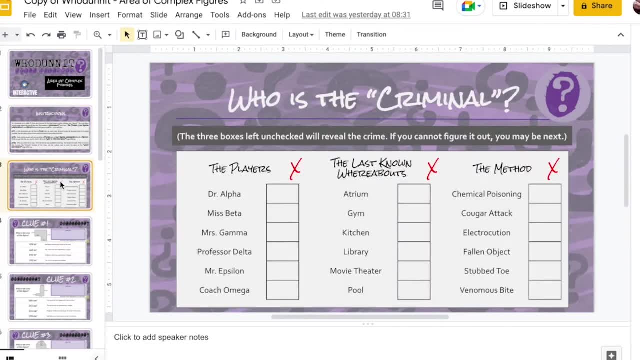 Obviously, they need to solve each of the questions, crossing out the incorrect answers and highlighting the correct answers. This page is the most important page of the whole activity, because this is the page where students are able to copy and paste the little Xs here into whichever box they think is the incorrect one And at the end, once they have, 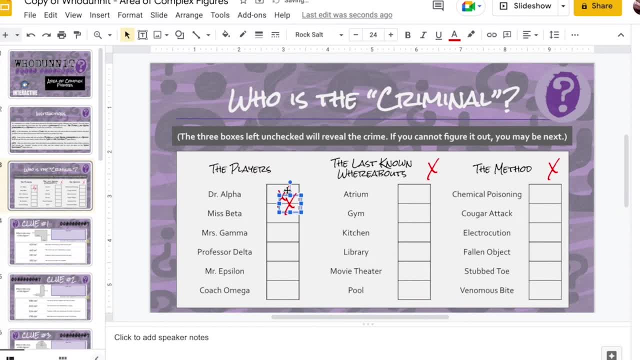 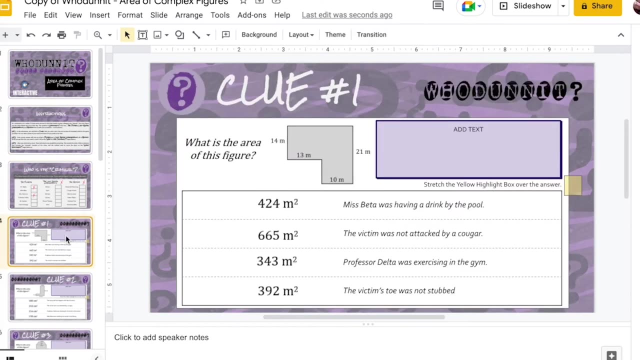 done the whole activity, then they should have it so that only one person from this or one player, one whereabouts and one method is left uncrossed. So, looking at the questions, this is our clue one. The question is: what is the area of this copy?